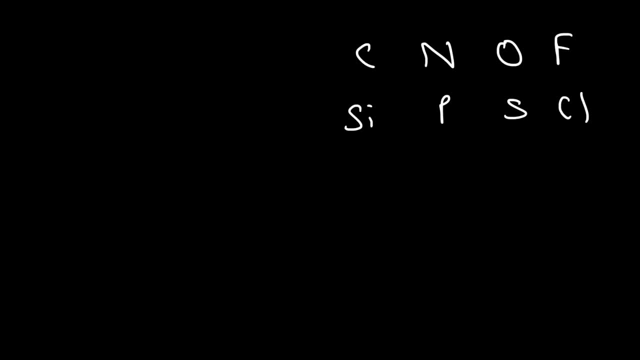 These elements. they can have what is known as the expanded octet. they can have more than 8 electrons. The reason why nitrogen can have more than 8 is because nitrogen is in the second row, And in the second row you have the 2s sublevel and you have the 2p sublevel. 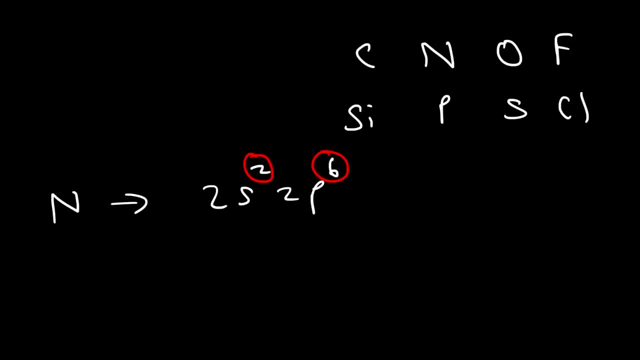 Notice that in the second energy level the maximum number of electrons is 8.. So that's why second row elements cannot have more than 8 electrons. It's just not possible. Phosphorus is in the third row, So in the third energy level you have the 3s sublevel, the 3p sublevel and the 3d sublevel. 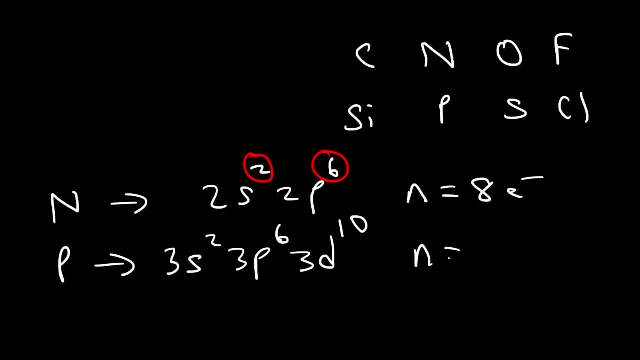 So therefore, in the third energy level you can have up to 18 electrons, And that's why elements like phosphorus, sulfur and chlorine, they can have expanded octets. So if they're the center atom they can have more than 8 electrons. 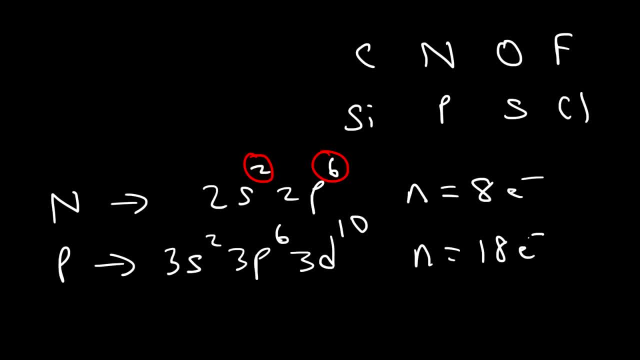 Sometimes you might see them have 10,, sometimes even 12.. So just keep that in mind. So anything that's in the third row or below can have an expanded octet, But the second row- elements like carbon, nitrogen, oxygen and fluorine- they cannot have an. 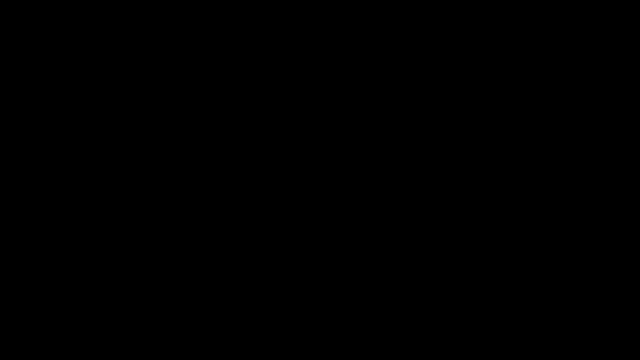 expanded octet. They cannot have more than 8 electrons. Now let's consider an example of an expanded octet: PCl5.. Go ahead and draw the Lewis structure of this substance: Phosphorus has 5 valence electrons and chlorine has 7.. 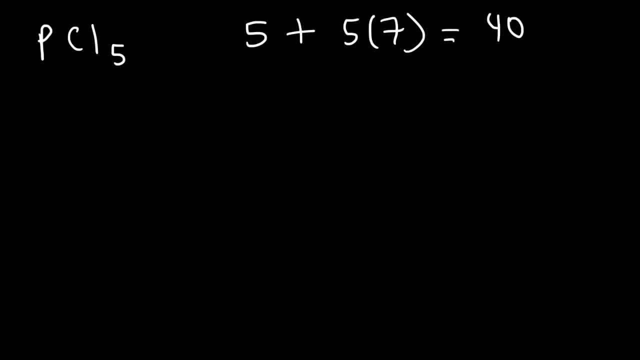 5 times 7 is 35, plus 5 is 40. And to calculate the number of lone pairs, it's equal to the valence electrons minus 8n divided by 2. So there's 40 valence electrons and n is the number of atoms. that is not a center atom. 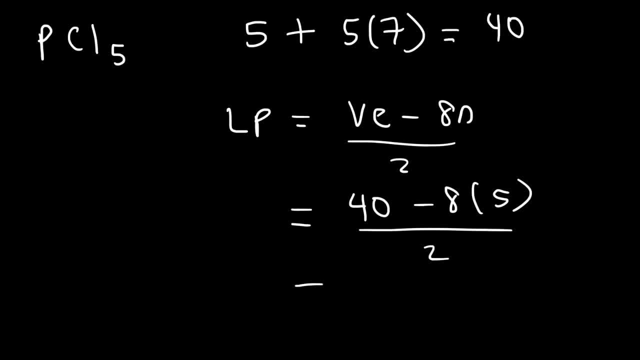 So n is 5 in this example. So 8 times 5 is 40.. So 40 minus 40 is 0.. So there are no lone pairs on a center atom. So to draw the Lewis structure all we need to do is put the 5 chlorine atoms around phosphorus. 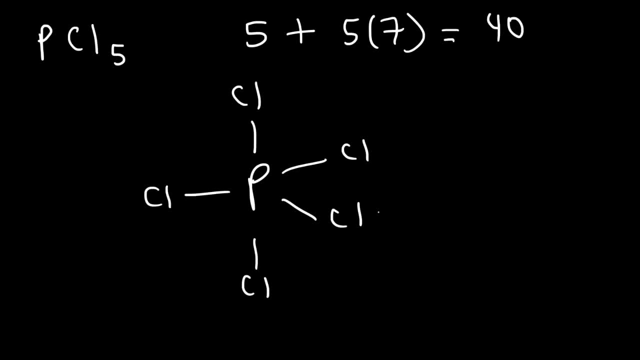 because there's no lone pair on phosphorus And, as you can see, phosphorus has more than 8 electrons around it. Because it has 5 bonds and each bond represents 2 electrons, it has a total of 10 electrons around it. 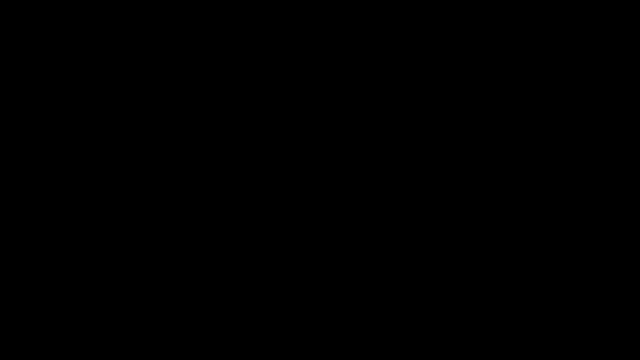 So it has an expanded octet. So let me give you another example. Let's use ICl5.. Go ahead and draw the Lewis structure for this molecule. So first let's count the number of valence electrons. Iodine has 7,, chlorine has 7.. 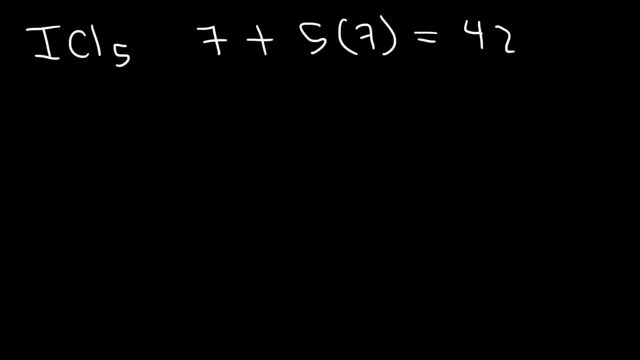 5 times 7 is 35, plus 7,, that's 42. Now the number of lone pairs is going to be 7.. This is going to be the valence electrons, which is 42, minus 8n. 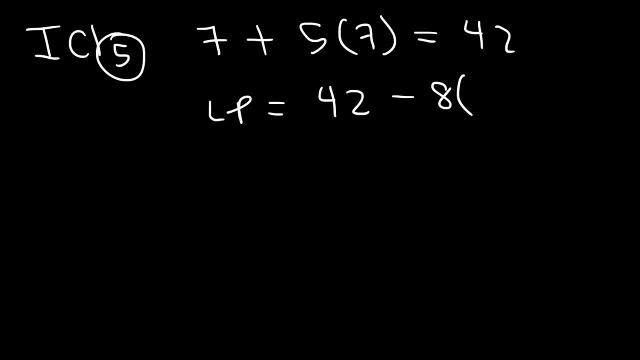 And n is the number of atoms. That is not the center atom, which is 5.. So 8 times 5 is 40, 42 minus 40 is 2.. So we have one lone pair on iodine, the center atom. 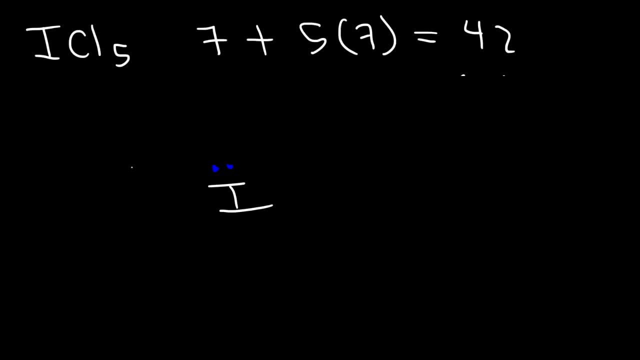 And there's 5 other chlorine atoms attached to it. And so this is the Lewis structure of iodine petachloride. It has a square, pyramidal molecular geometry And, as you can see, it has an expanded octet. It has two, four, six, eight, ten, twelve electrons around it. 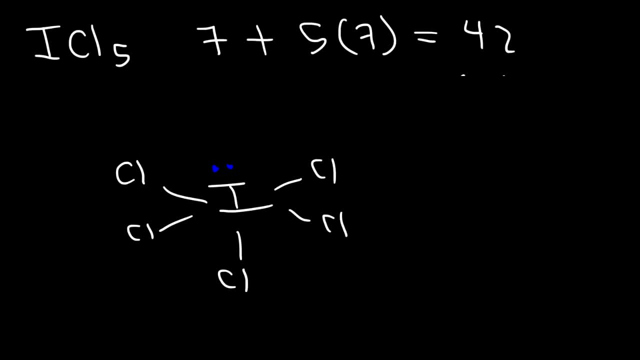 Hi, alltums, Your signatures, Your globally Captivated approximately 50 states examples that violate the octet rule, And this occurs when a molecule has an odd number of electrons. So let's consider nitrogen monoxide: Nitrogen has five. 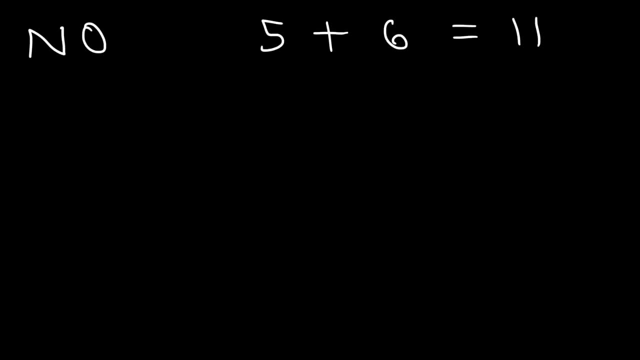 valence electrons and oxygen has six, So the total is 11.. So how can we draw a Lewis structure in which we have 11 electrons? The first thing I like to take into account is the number of bonds that certain elements like to form. So let me 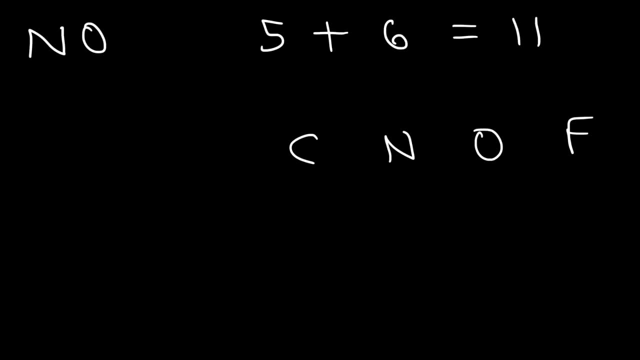 just give you a quick review of how to determine that Carbon has four valence electrons, Nitrogen has five, Oxygen has six, Fluorine has seven. Now elements on the right side of the periodic table. they like to acquire electrons, So carbon. 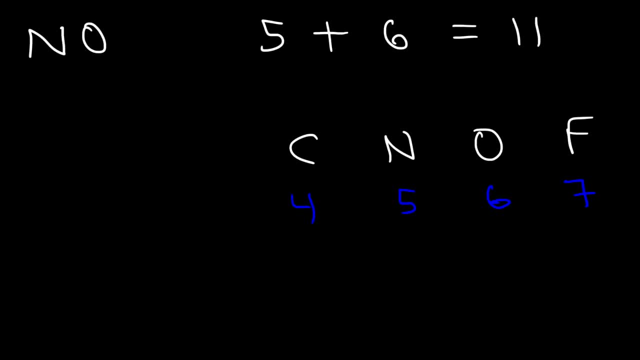 wants to have eight. It needs to get four more electrons in order to have eight. So carbon likes to form four bonds to get those four electrons that it needs. Nitrogen has five valence electrons. It needs three more to get to eight. So it 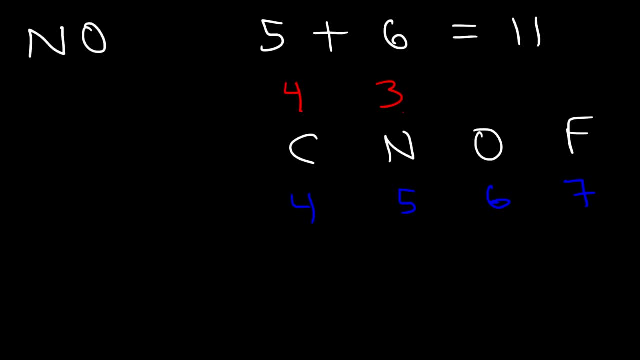 likes to form three bonds to get the three electrons it needs. Oxygen likes to form two bonds. Fluorine likes to form one. Now, on the left side, these elements like to give away electrons instead of acquiring electrons. Boron has three valence electrons, So it forms three valence electrons, So it forms three. 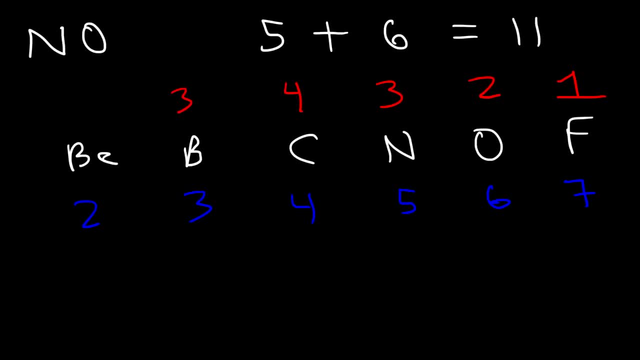 bonds to give away those three electrons. Beryllium has two valence electrons So it likes to form two bonds to give away those two valence electrons And so knowing that can help us to get a good idea of how to draw the Lewis structure. 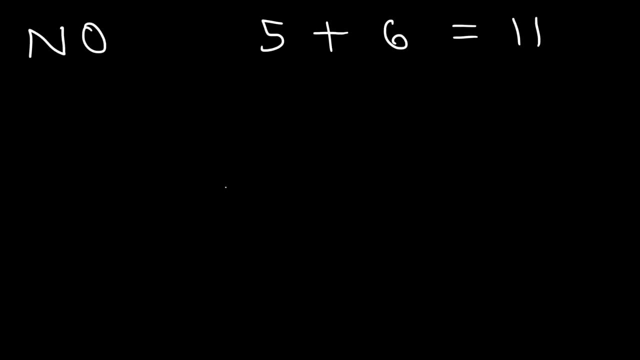 for NO. So now let's go ahead and draw. NO Now. nitrogen likes to form three bonds, but oxygen likes to form two. This molecule is either going to have two bonds or three bonds, So let's start with two. We need a total of eleven electrons. Right now we have four Every. 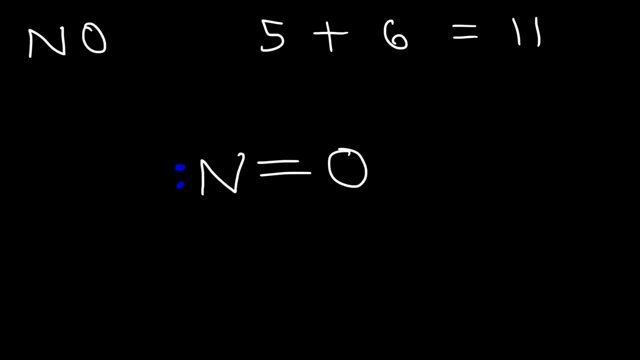 bond represents two, So now we have six, and now we have eight, Now we have nine, Now we have ten. So who's going to get the last electron? There's two ways in which we can draw: We can give it to oxygen, or we can give oxygen to oxygen. 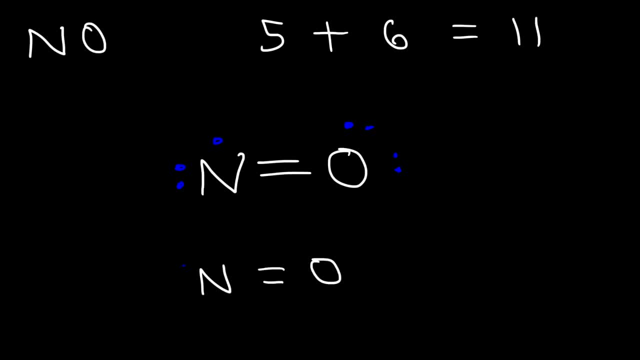 The last electron to nitrogen. As you can see, either way you draw, one of these atoms will have an incomplete oxide. In the first example, oxygen has eight electrons: Two, four, six, eight. So its oxide requirements are satisfied. But 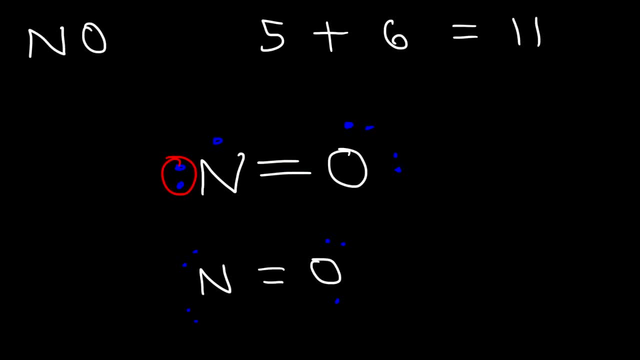 nitrogen has seven, Two, four, six, seven. In the second example, nitrogen has eight, but oxygen has seven, Two, four, six, seven. So regardless of how you structure this molecule, you're going to have an element that has an incomplete. 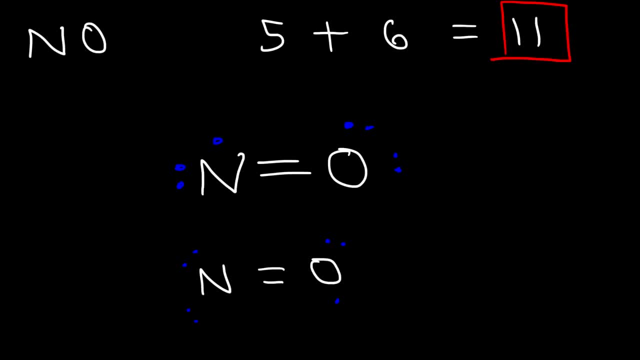 octet. So anytime you have an odd number of electrons, the octet rule will be violated. There's nothing you can do about it. It's just based on the numbers that you have. Now, which way is the best way to draw this structure? Should? 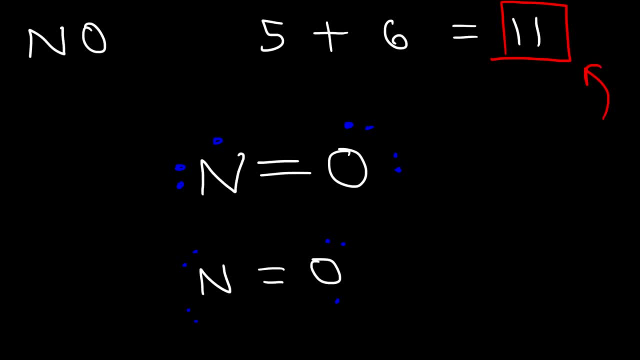 oxygen have eight or should nitrogen have eight? Now, which element is more electronegative? Oxygen is more electronegative than nitrogen. Electronegativity increases as you go up and to the right, towards fluorine, and because oxygen is closer to fluorine than nitrogen on a periodic table, oxygen is more electronegative. 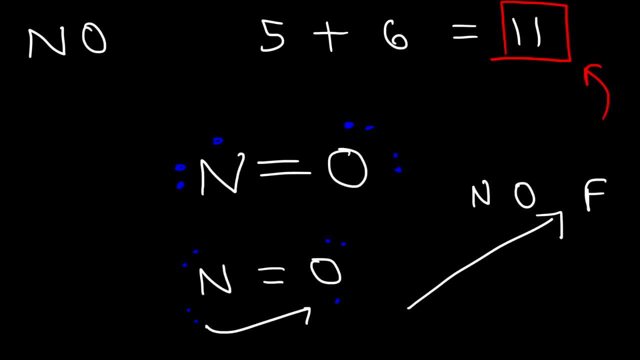 So oxygen is going to take away that one electron, and so this is going to be the most stable Lewis structure out of the two that's listed. Now let's try another example in which we have an odd number of electrons. Go ahead and draw the Lewis structure for NO2.. 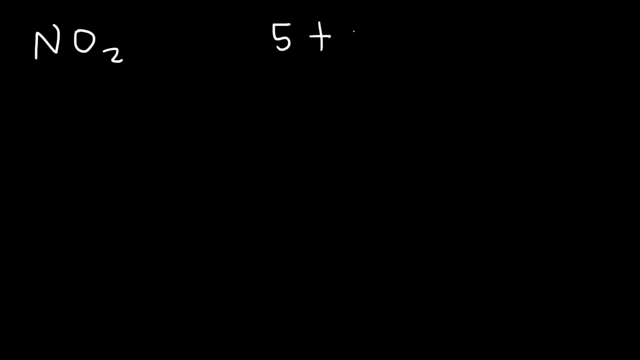 So nitrogen has 5 electrons, oxygen has 6.. So this is going to be 12 plus 5, so that's a total of 17.. Okay, So chances are nitrogen is going to be the center atom, since nitrogen can form more. 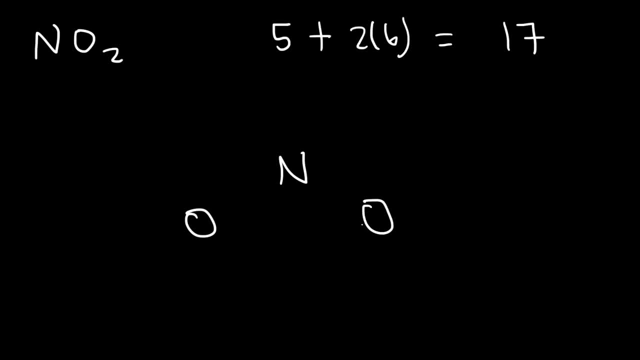 bonds than oxygen. Oxygen likes to have two, but nitrogen likes to have three. But when you have an odd number of electrons, something's going to be lacking. So each bond needs at least one single bond. Now if we calculate the number of lone pairs, let's see what's going to happen. 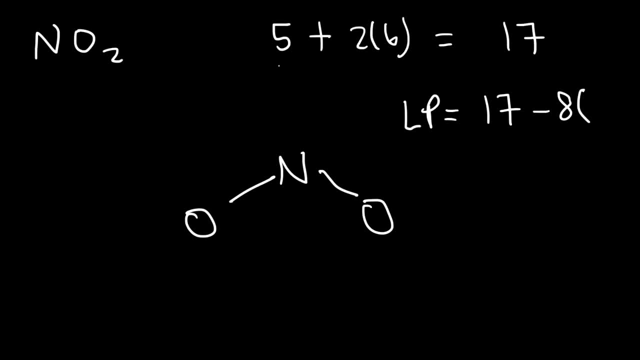 So we have 17.. We have 17 valence electrons minus 8n, and it's 2.. There's two atoms that are not center atoms divided by 2.. So 17 minus 8 times 2, that's 16.. 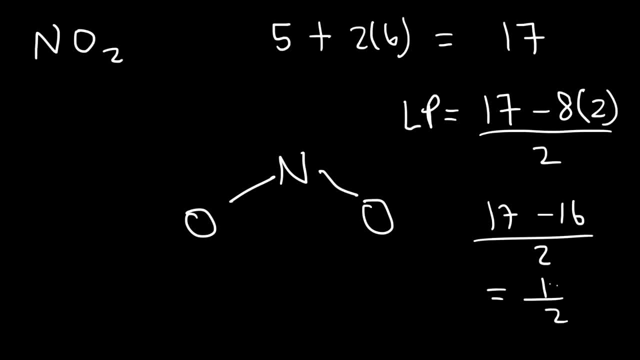 That's going to be 1.. So what we have is half of a lone pair. Half of a lone pair is one electron. So now, at this point, we have a total of 5 electrons: 2,, 4,, 5..